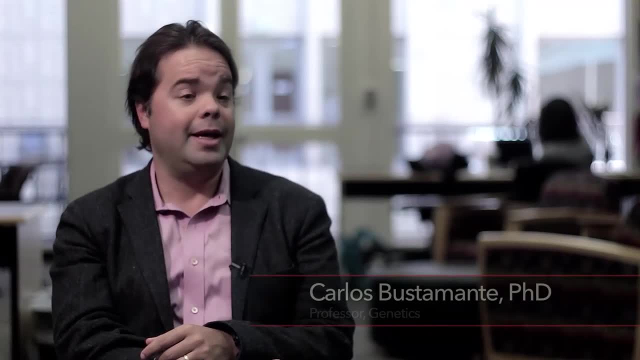 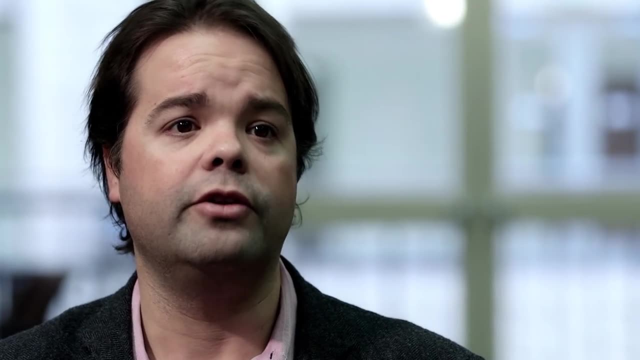 biomedicine in the 21st century. When we think about big data, we think about all the excitement, of all the different data sources, But ultimately it's really sort of the discipline of data sciences that underlies the methodology, the tools, the 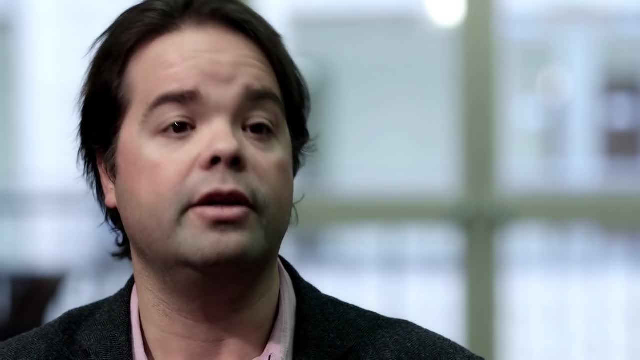 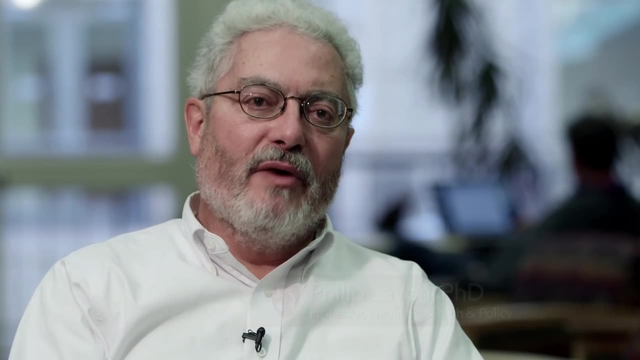 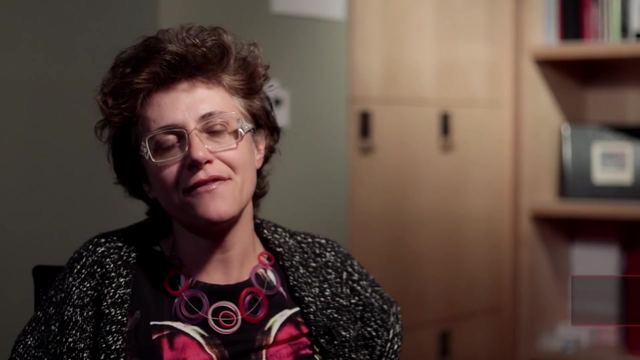 approaches the way we synthesize that information to really extract knowledge from data. Data science is what statistics became in the 21st century, when other people besides statisticians began taking it seriously as a discipline, But it also has an emphasis on the fact that we use data to generate. 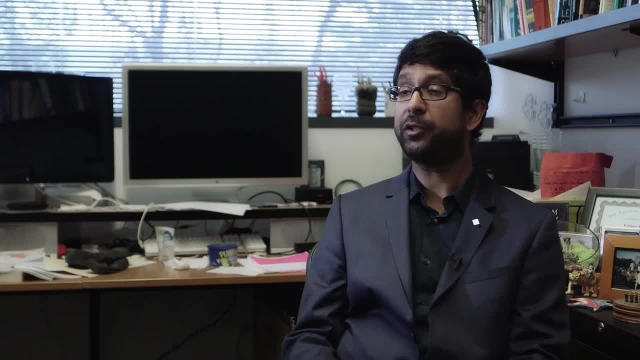 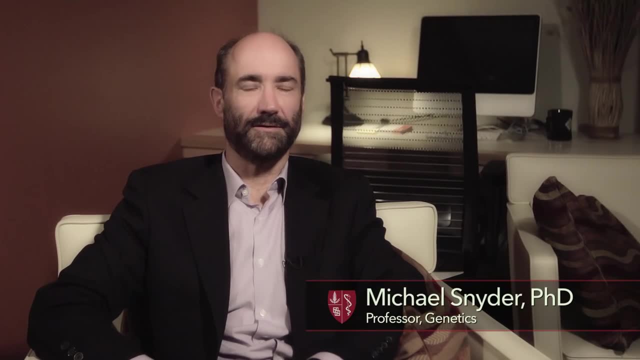 our hypotheses on how the world looks. So why should the average person care about data science? Well, you know it's interesting to think about all the impacts that could come. We can learn so much about you, your DNA, billions of other measurements that we can make, both on your molecules, to understand your 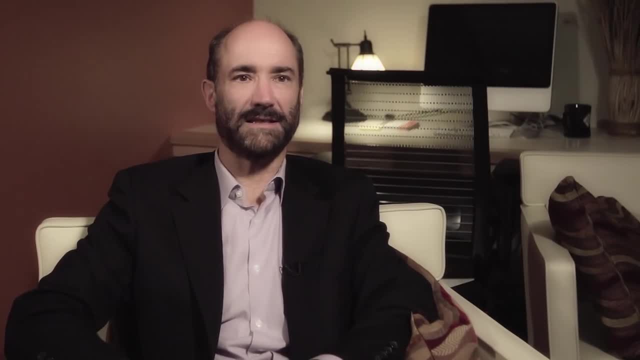 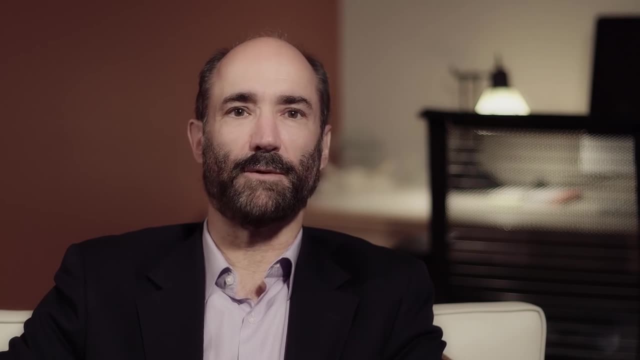 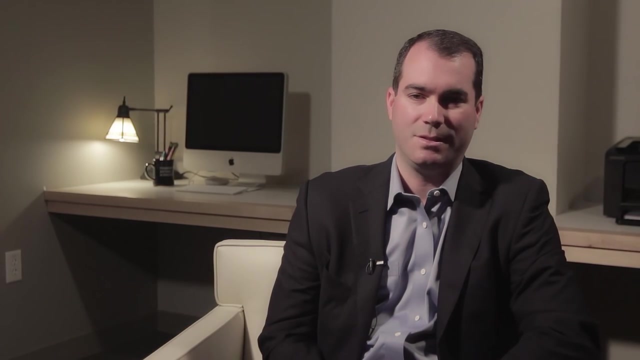 health state, as well as all the things you do in terms of your activity. So the goal is really to make these measurements and understand people as soon as problems arise Again, maybe before they even realize it. As the father of a child that has benefited directly from whole genome sequencing, I 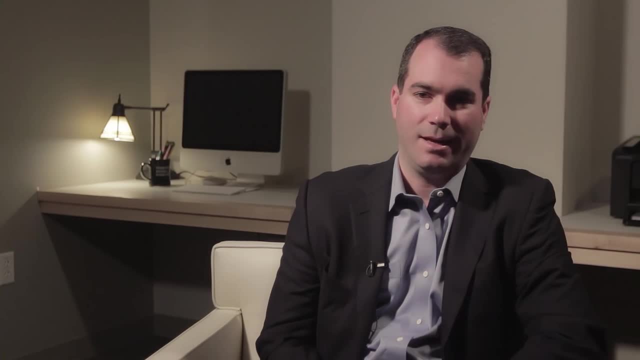 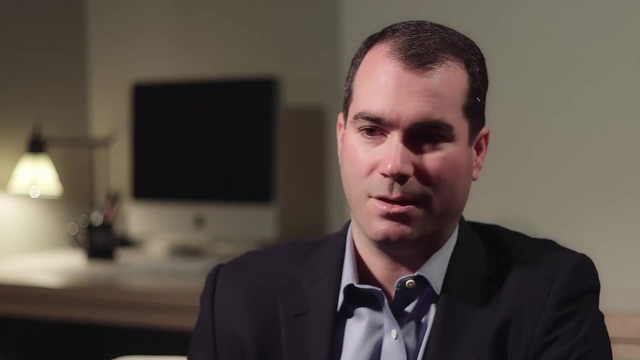 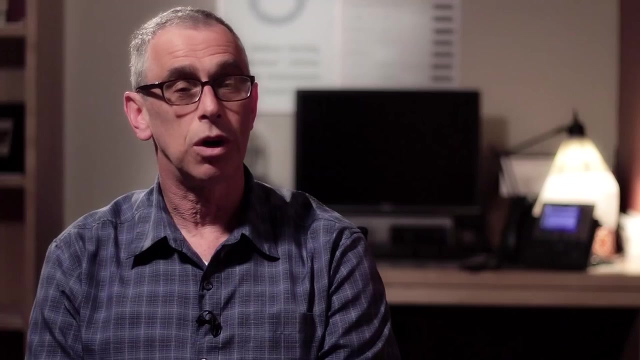 can say unequivocally that a diagnosis has given us much hope and a lot to look forward to and a lot to work on. Can we use information about a patient's genome or about their exposures out in the world to make precise drug prescribing decisions, And can we use information to figure out how we can? 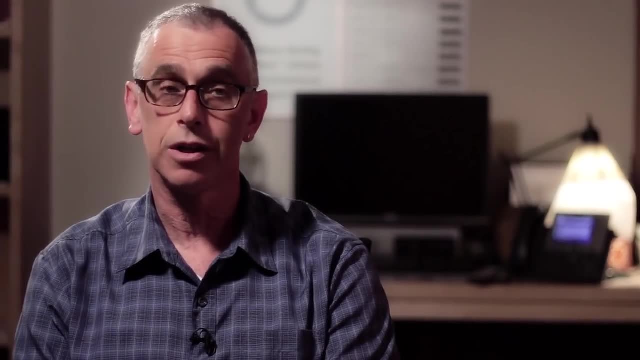 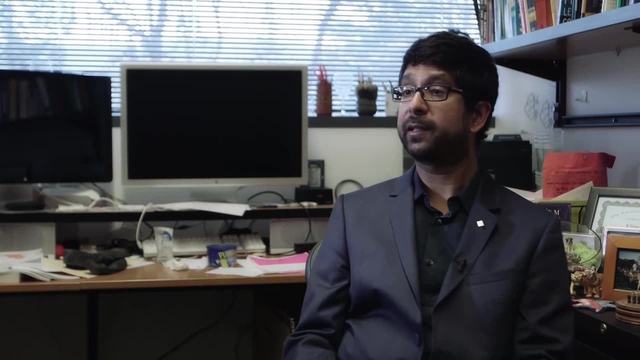 combine medications, perhaps even using old drugs to treat new diseases. We actually use large-scale machine learning to try to understand how to better design drugs, And it's allowed us to make impacts in many different areas, especially basic biophysics and drug design in the areas of. 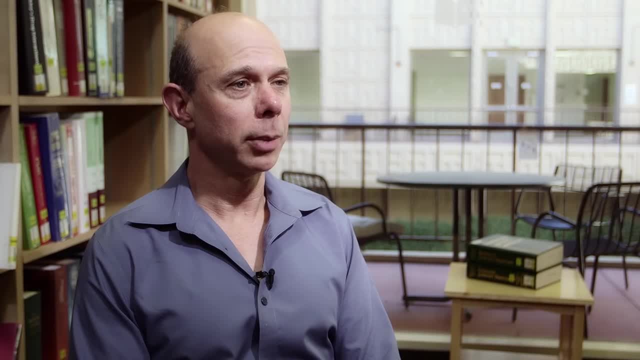 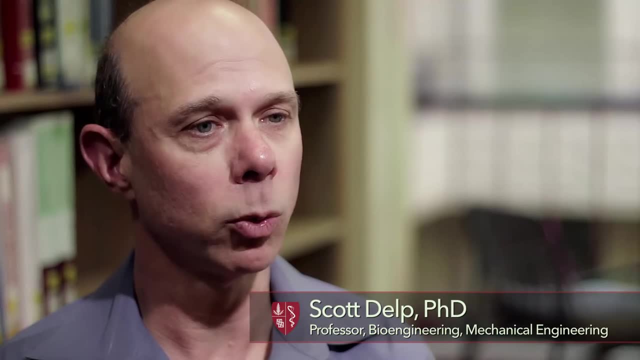 Alzheimer's and infectious disease. One of the things we've learned using big data is that how to make better surgical decisions, And we've made discoveries about which surgical procedures, for example, will lead to greater mobility in people who have cerebral palsy In our 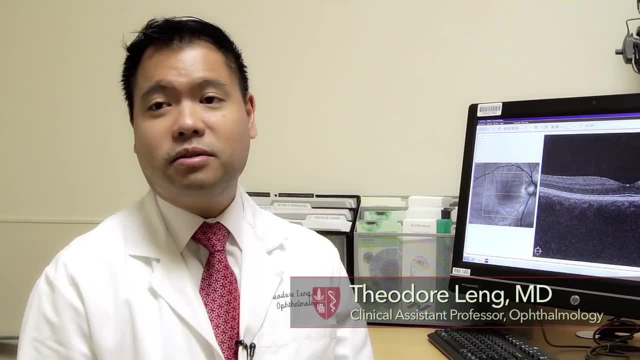 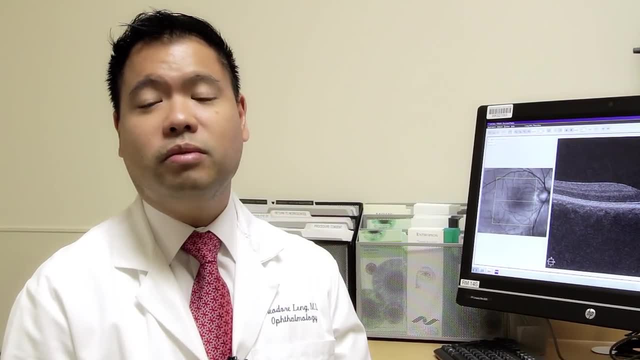 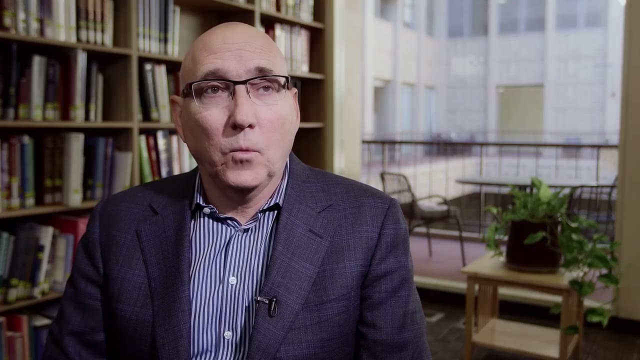 research. what we've done is taken data from retinal scans, which are acquired at every visit here for patients with macular degeneration, and created a mathematical model in order to be able to predict which patients might be getting worse and which patients should be safe from progression. We're looking 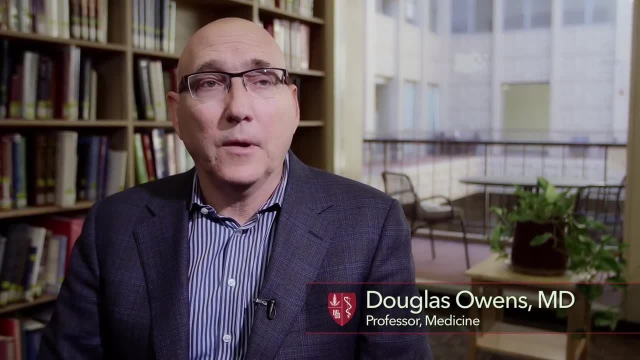 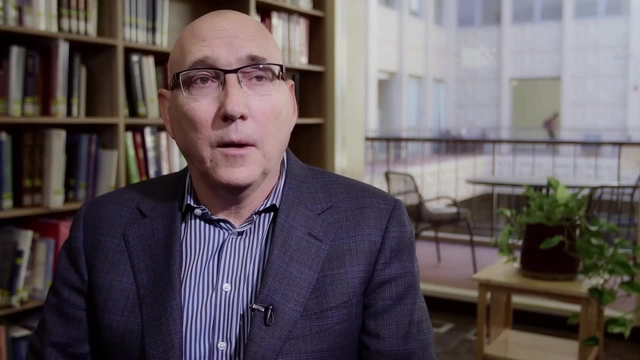 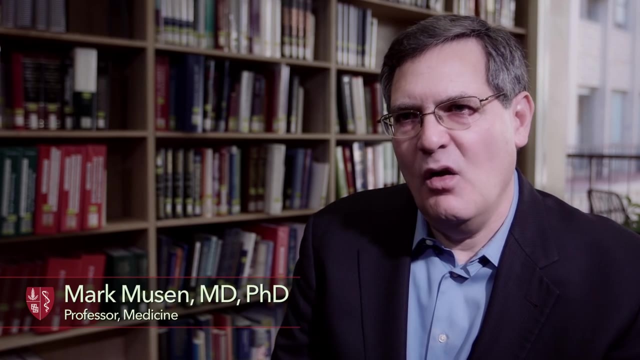 at how the big data about where people come from, where they live, can help us in terms of outreach and help us in terms of improving the care that people with hepatitis B get. Stanford has a lot of exciting advantages in data science. We're all on. 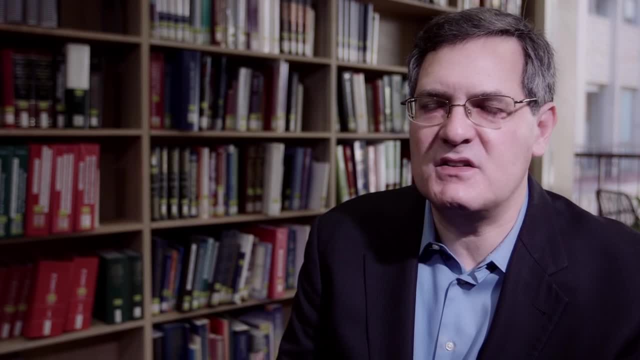 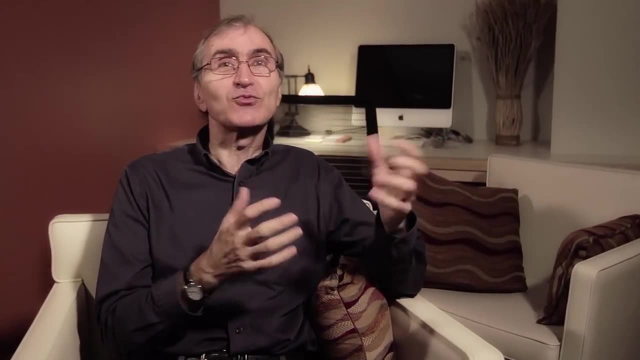 the same campus. people who do work in informatics and computer science, people who understand the ethics and the security issues related to big data. We've been doing data science at Stanford for many years. What's new these days is bringing together the scientists that are generating data with the ones. 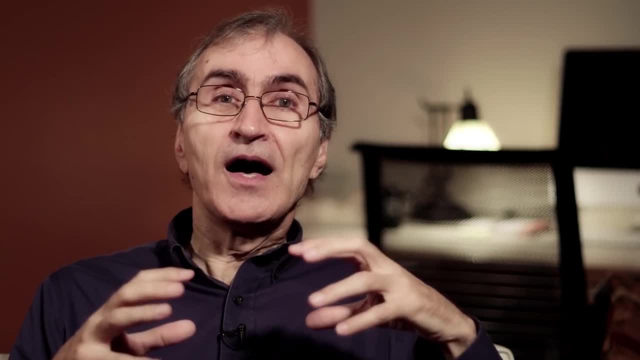 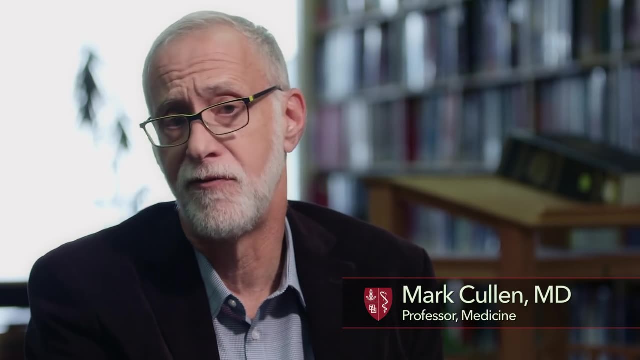 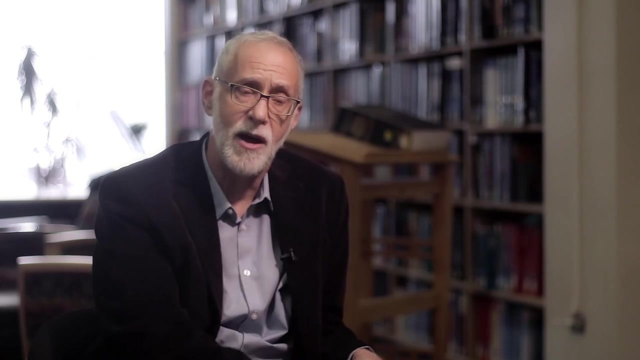 that understand how to analyze the data to make new discoveries. We've got people doing remarkably innovative work across the spectrum, ranging from very basic biology all the way out to the studies of physical environment, social environment, public health and so forth. Stanford School of Medicine has arguably the best biomedical research program in. 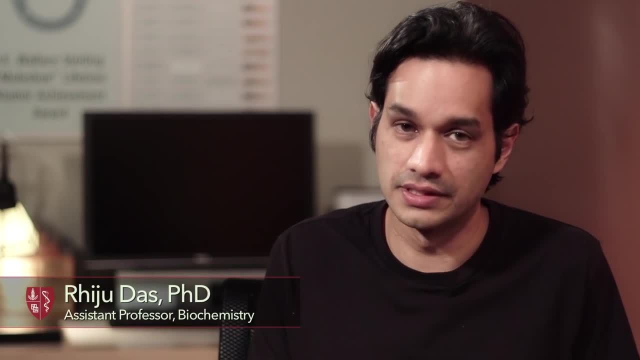 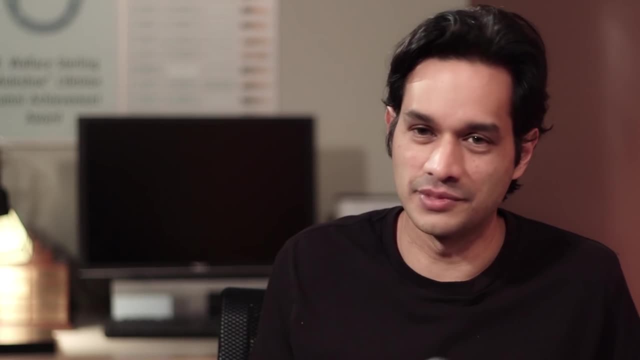 the world right next to Stanford Hospital and the world's leading hospitals, And the cool thing is that all of our labs and groups in computer science, engineering, physics, biology, biochemistry- we're all right next to each other. This is really something that brings together all of Stanford and all of 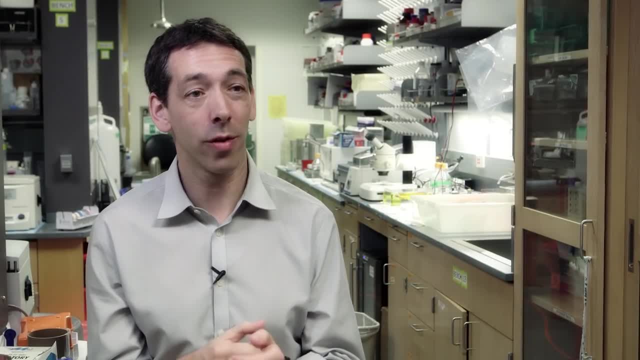 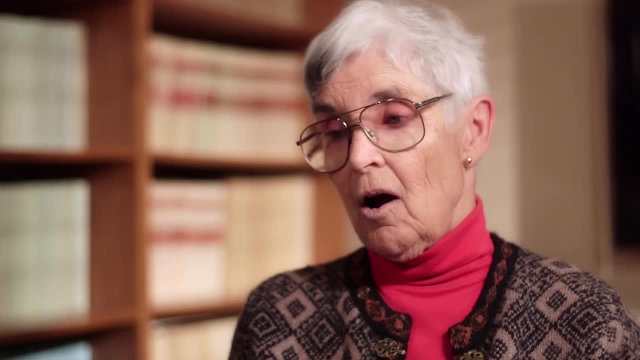 Stanford's strengths, And then we can reach outside of the Stanford campus to our neighbors who are in the technology industry, who've been using data science to transform the world around us. Oh, it's going to be very, very exciting because I think we're going to be making 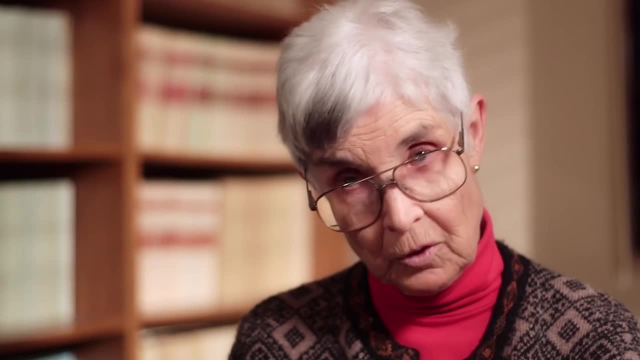 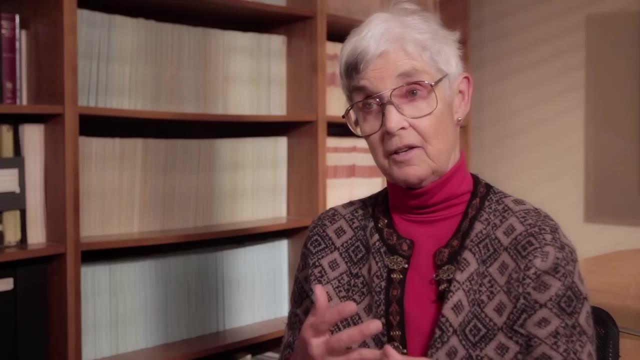 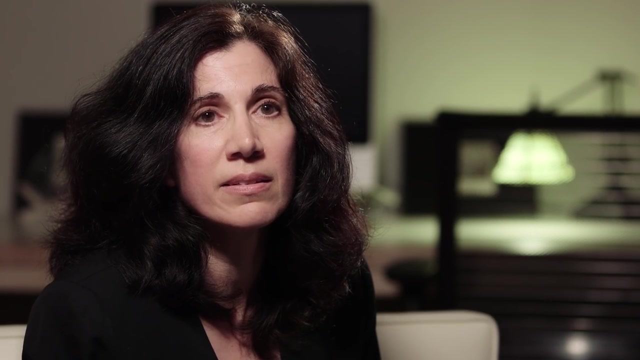 more and more discoveries about how individuals can prevent disease and restore their health and therefore their quality of life. Looking into the future, I see us as a more informed society. I see scientists working in domains that they didn't expect to work in, because they have. 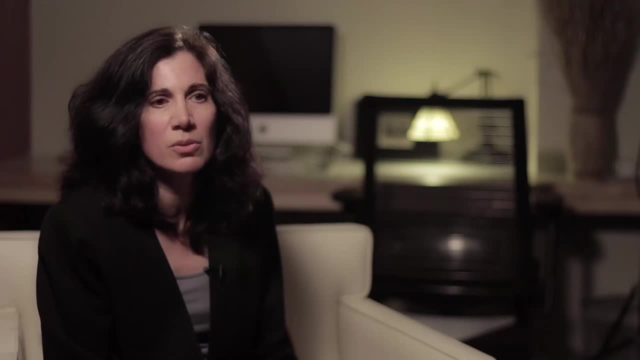 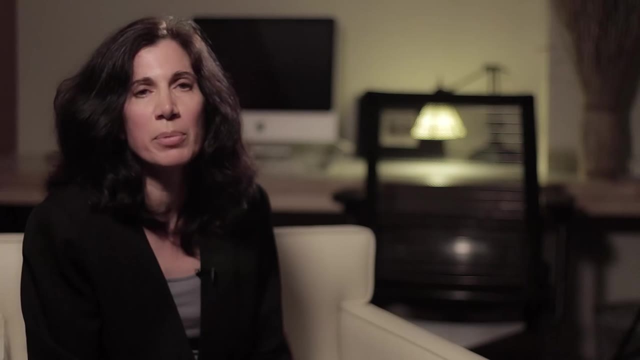 access to data they didn't have access to before, And I do see that that's going to help the individual, because I do believe this information is going to translate into decisions that will empower the individual to make better choices. I think that big data could serve as a